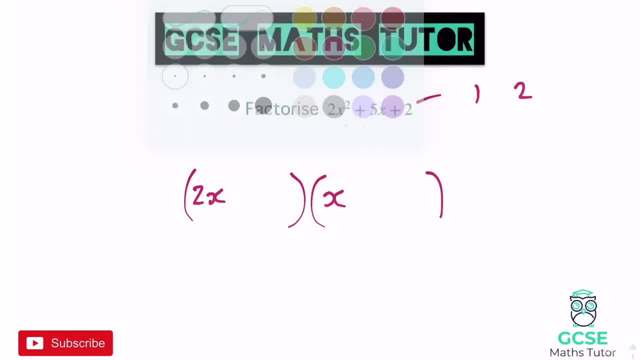 numbers in the bracket is going to end up getting multiplied by 2, because we have this 2x at the start of this first bracket. So that means when I look at this number 1 and this number 2, I've got to think: well, one of them is going to have to double. and if 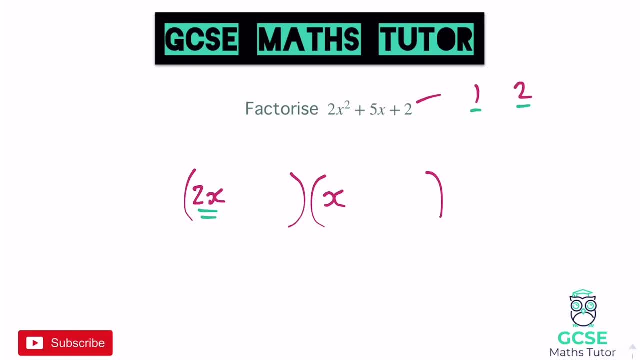 one of them's going to double, and I tend to do this in my head, but I'll write it down. we could either have 1 not doubling, and 2 doubling, which would give us 4, or we could have 2 doubling, which would give us 2,, and 2 not doubling, which would give us 2 again. 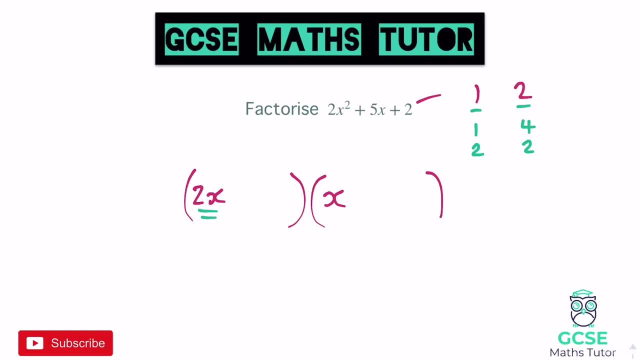 So I've got two options from this pair. I've got 1 and 4, or 2 and 2.. And I'm going to try and make 5 in the middle. Now I can't make 5 out of 2 and 2, so I know. 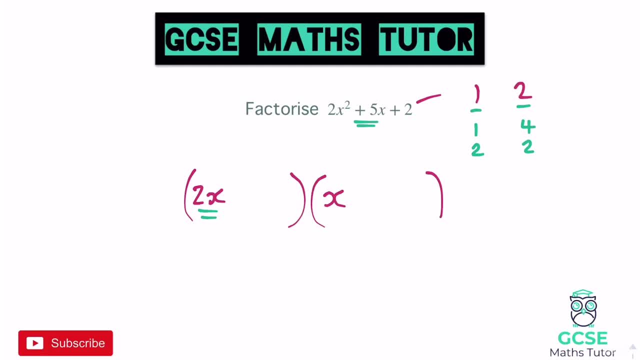 it's not 2 and 2, but it's going to be 1 and 4.. OK, 1 and 4 can make 5, so I've just got to think: OK, well, this is the pairing I'm going. 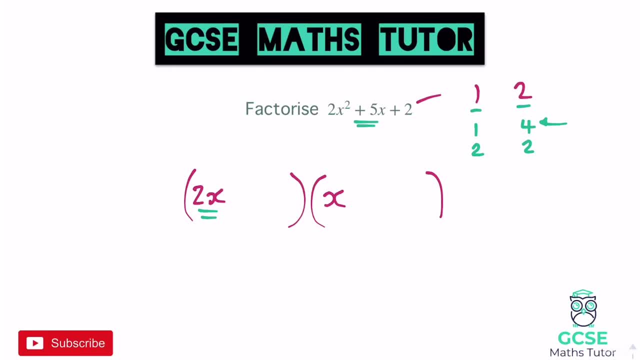 to go for 1 and 4, which number do I want to double? That's the 2 sitting above it. so if I want the 2 to double, I want the 2 to go in the other bracket and I want the 1 to go in the first bracket. being careful not to write. 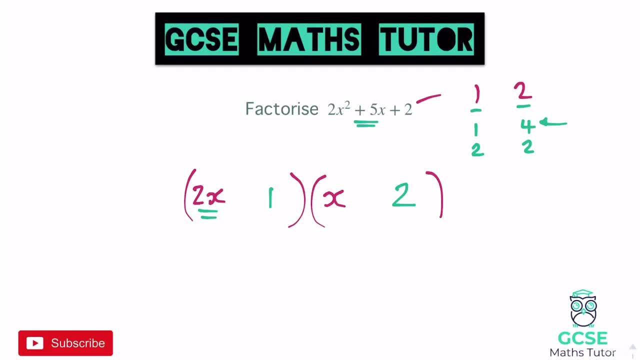 the 1 and 4 there, but to write the original 1 and 2. Now it's all pluses, it's all positives, so it's just pluses And pluses. in both of these we can have a look at some with some negatives, but that 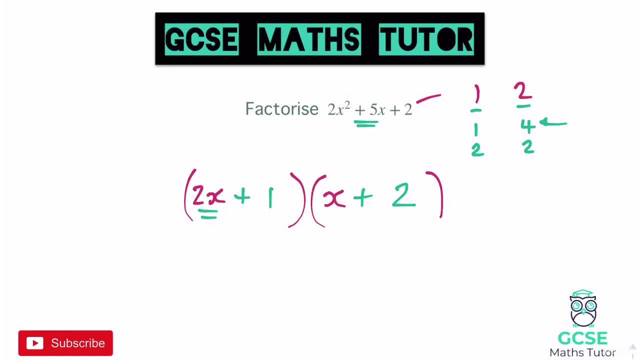 would be that factorised there. But again, just using that logic, write down your factors and think: OK, well, which one's going to double or triple or whatever the x squared value we've got in this question? OK, let's have a look at another one. 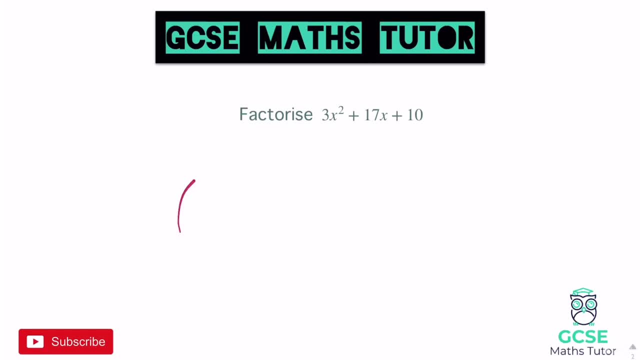 OK, so we've got a 3x squared in this one, so it's a very similar process. In order to get a 3x squared, we would have an x and a 3x, So if I put those in to start with 3x. 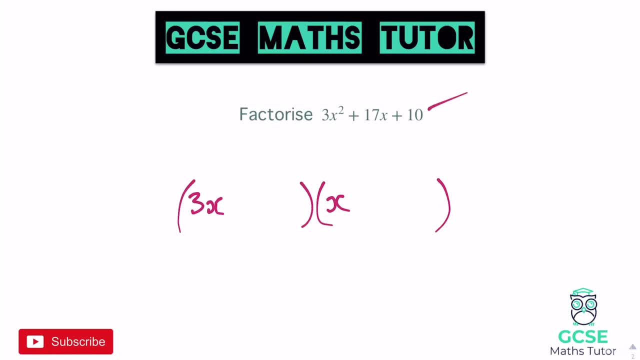 and x. Same process with the 10. here let's write down what the factors are. we've got 1 and 10.. Or we could have 2 and 5.. Now, this time, because there's a 3x in this bracket, that means one of them is going to. 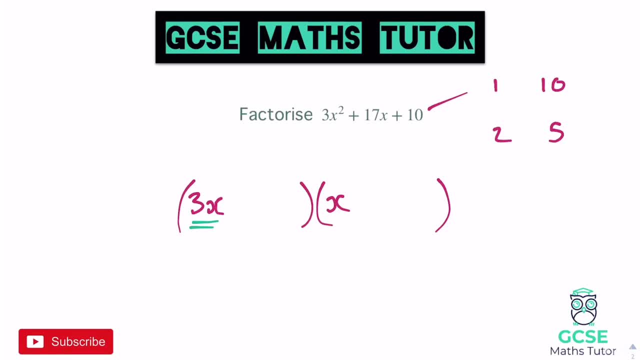 triple or get multiplied by 3.. So looking at the first one there and you might be able to just do some of these in your head, but I could have the 1 tripling to make 3, and that would be 3 and 10.. Or 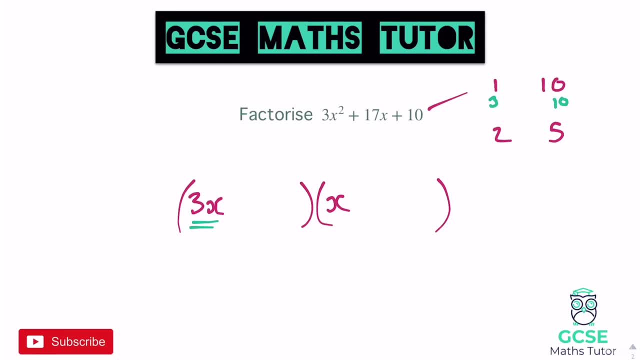 I could have the 10 tripling and that would be 30 and 1.. Now, I'm not going to make 17 out of 3 and 10,. I'm not going to make 17 out of 30 and 1 either. 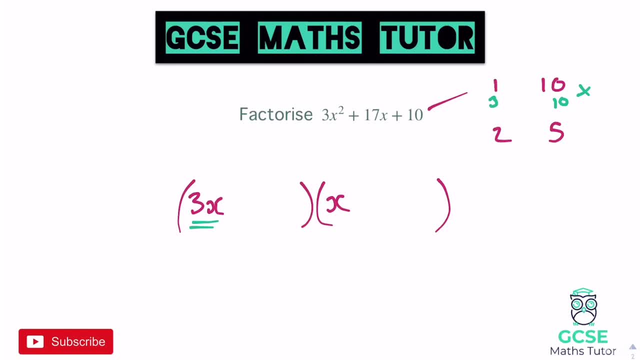 So it's not going to be 1 and 10, so let's have a look at the 2 and the 5.. So I could have the 2 tripling to make 6 along with a 5, or I could have the 5 tripling. 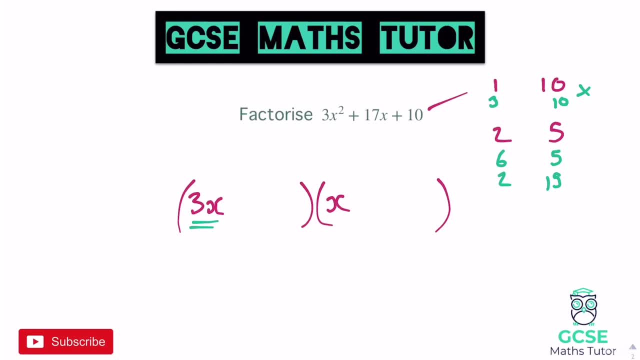 to make 15 along with the 2.. So there are my options there, just tripling one of them. Now, I'm not going to make 17 out of 6 and 5, but I can make 17 out of 15 and 2.. 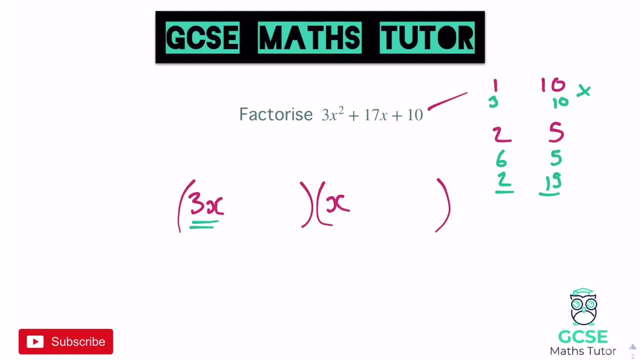 It's all positives again, so it doesn't matter which symbols we've got. we know it's going to be positive in both. I've just got to make sure that I get that 15 appearing in the other bracket, so that means putting a 5 in the second bracket. 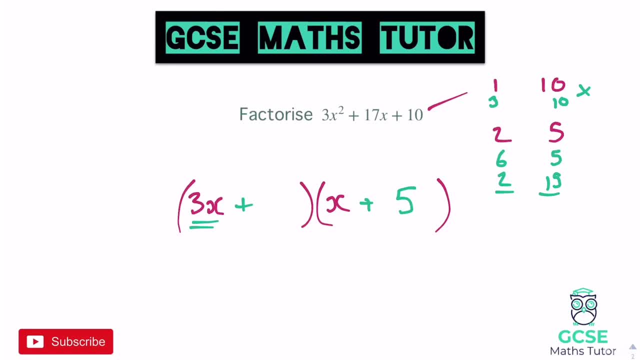 That's simple, second bracket. and then when you were to expand that, we'd get 15 and we might expand this one and the two- the original two goes in the other bracket and again, if you're not sure, just make sure you go about expanding it. so, 3x times x gives you 3x. squared, 3x times the 5 gives us 15x. 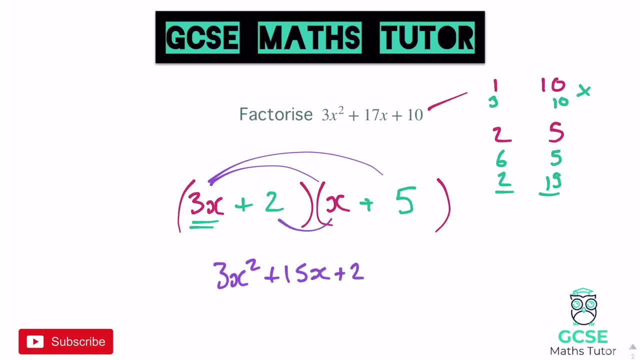 2 times the x gives us 2x, and then 2 times 5 gives us 10. so it's a nice little check there that you can do. at the end, obviously, you just tidy these up and you see where that 17x comes. 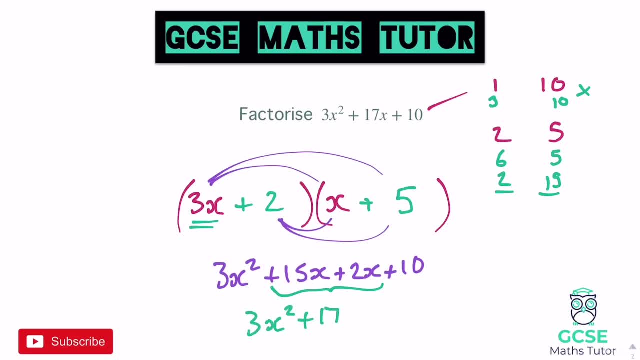 from that we wanted. so 3x squared plus 17x plus 10, and again, you know, if it doesn't expand correctly or you're not sure on it, you can always go back and have another go and you can use a bit of trial and error. but just think about it logically, with your factors to the side. so we've got one more. 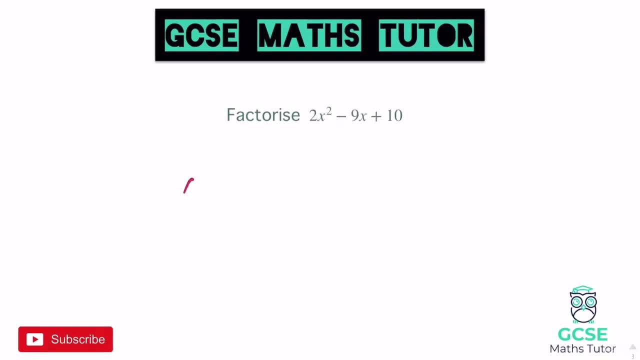 okay, so introducing some negatives. same process, though we'll stick 2x in one bracket and x in the other, as we've got a 2x squared, and again writing down the factors of 10, so 1 and 10 or 2 and 5. 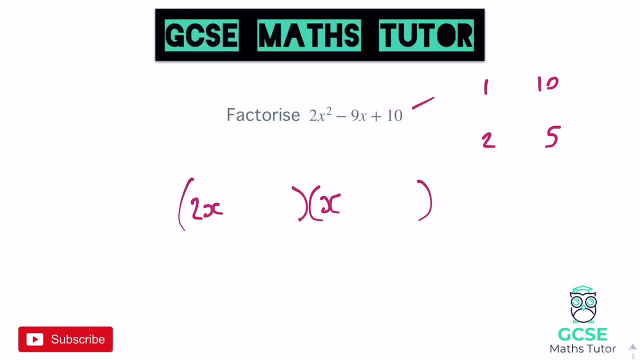 now Again, one of them is going to double, so we could have 2 and 10, or we could have 1 and 20.. Are we going to be able to make 9 out of either of those No 2 and 10,? we could make 8,, we could make 12,, but we can't make 9.. 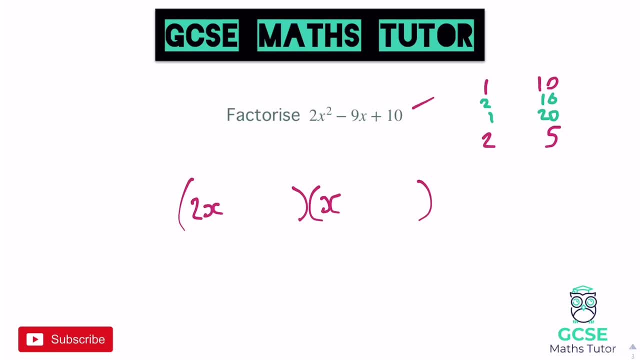 And then 1 and 20, we could make 19 or 21,, but we can't make 9.. So it's not going to be 1 and 10 at that, which means it's going to have to be the 2 and the 5.. 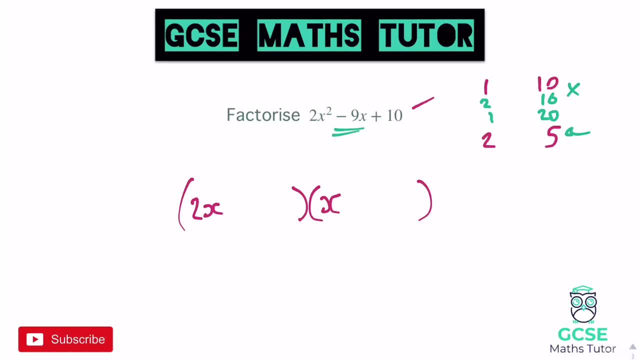 We've got to be a little bit careful here, because we've got negative 9 in the middle. so we are trying to make negative 9,, but similar process to when we were factorising before. So let's double one of them, so we could have 4 and 5, or we could have 2 and 10.. 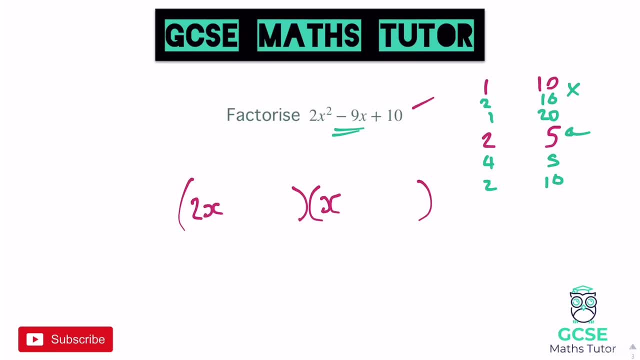 There we go, just doubling one of them. So again we're trying to make negative 9, so it's going to have to be 4 and 5.. We can't make 9 out of 2 and 10, but we can out of 4 and 5.. 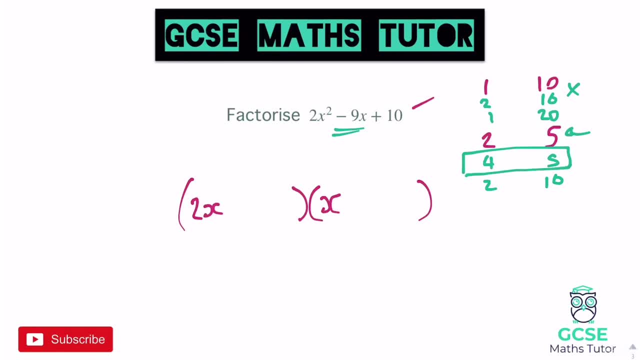 We've just got to figure out, OK, well, which one of these needs to be negative. And actually, looking at it, look, we've got a positive 10 at the end, so they're both going to have to be negative. 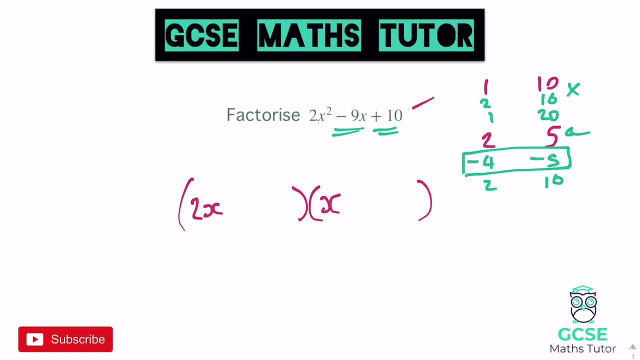 So it's going to have to be negative 4 and negative 5.. So I just want to make sure that that number above the negative 4, the 2, goes in the bracket that's going to be doubled. So on the right-hand side there we want negative 2.. 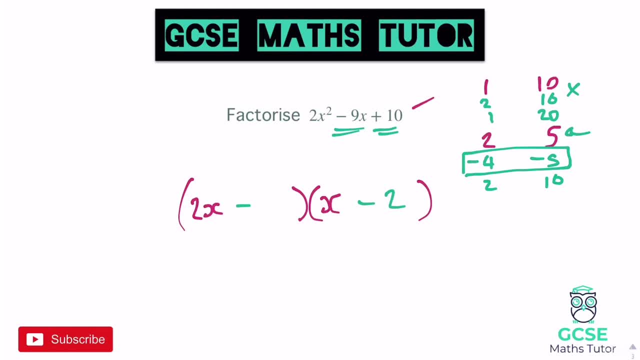 That's going to allow us to get negative 4.. And on the left bracket, there we'll put the negative 5.. And again, you can just expand that to just double-check. So 2x times x is 2x squared. 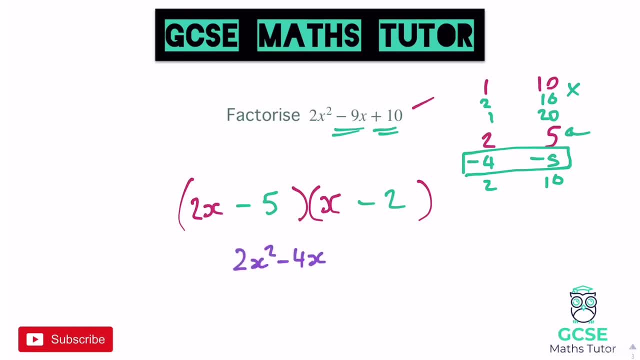 2x times negative. 2 is negative. 4x Negative 5 times x is negative 5x. And then negative 5 times negative. 2 gives us the positive 10 at the end there And tidying that up, look, these two here do make my negative 9.. 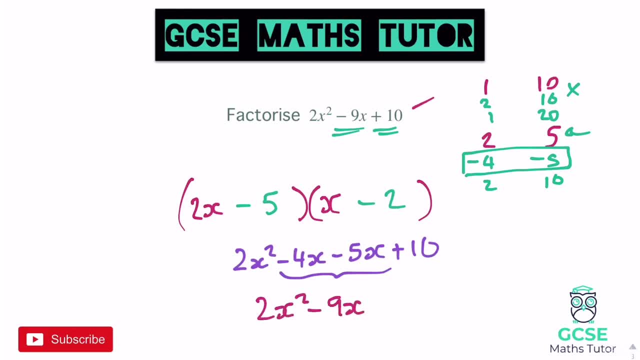 And we get 2x, 2x squared, minus 9x plus 10, and it matches what we were looking for. OK, so time for you to have a go. Here they are. So here's four questions. Pause the video there. 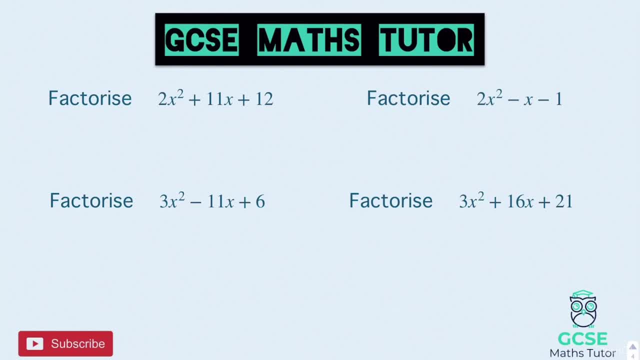 Have a go and we'll go over the answers in a sec. OK, so factorising these then So factors of 12, we can have 1 and 12,, 2 and 6, or 3 and 4.. 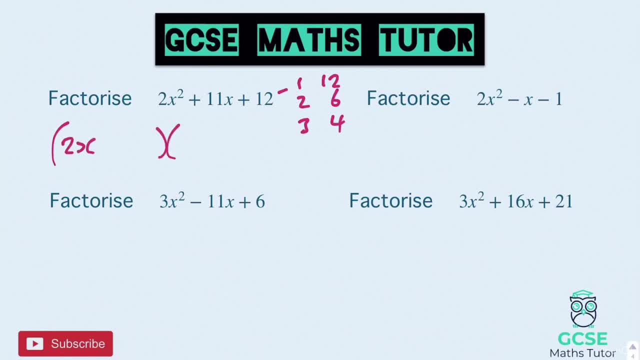 And in my brackets we're going to have 2x and an x And we're trying to make 11, so let's just look through the numbers. I'm just going to do them in my head. So I can't make 11 if I double anything in 1 and 12.. 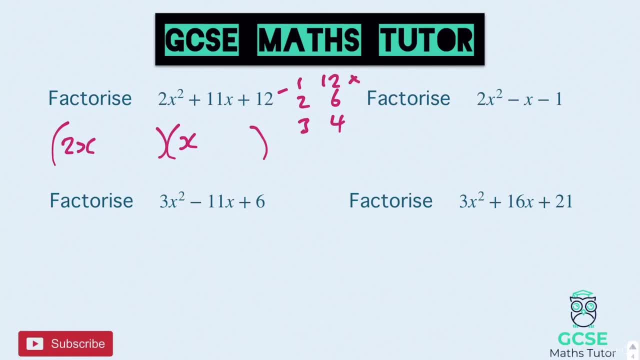 So it's not those. I could do 4 and 6, which isn't going to make 11.. Or I could do 2 and 12.. That's not going to work either, So it must be the 3 and the 4.. 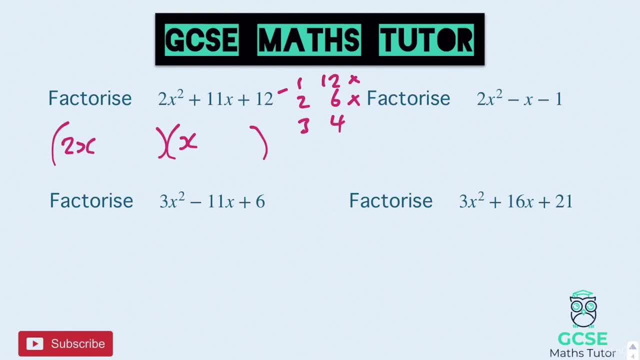 So double 3 is 6, and 4 would make 10.. That doesn't work. But double the 4 to make 8 and add 11. That would work, So doubling the 4.. So we'll stick the 4 over here and the 3 in here. 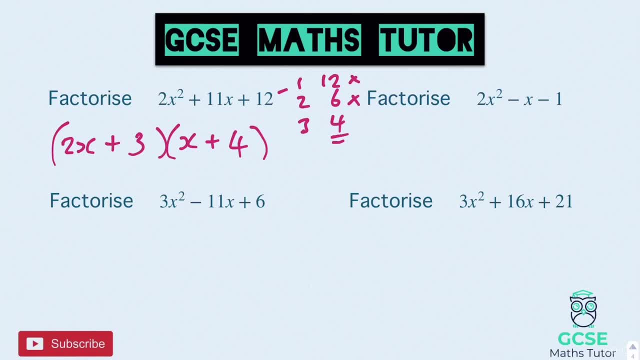 And they're all positive for this one. so that's quite nice, Right on to the one below. So 3x squared. So we're going to have a 3x and an x And again one of my factors is going to triple here. 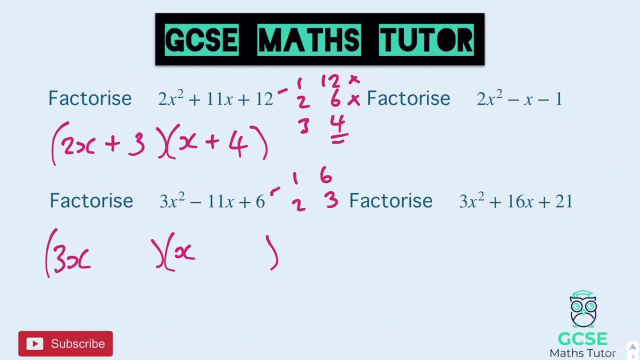 So 1 and 6,, 2 and 3.. How do I make 11 if one of them triples? Well, I don't want 1 and 18, and I don't want 3 and 6.. So they're not going to work. 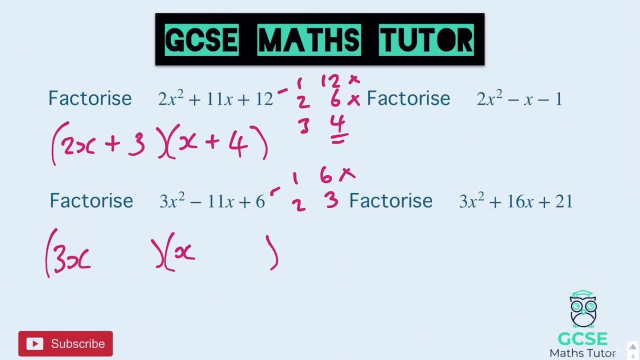 So it's going to have to be 2 and 3.. So I could have 6 and 3,, which would make 9.. Or I could have 2 and 9, and I can make that out of 11.. So I want my 3 to be tripled to make 9.. 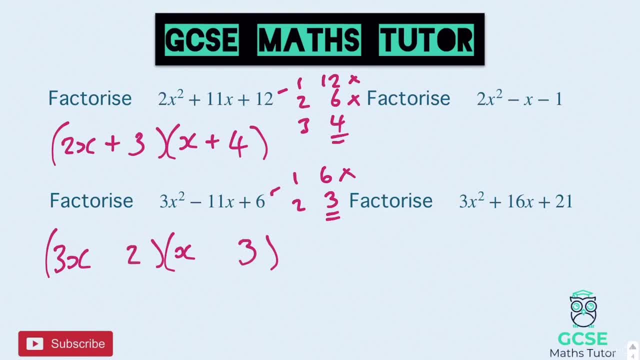 So let's stick the 3 in here and the 2 in here, And again we're trying to make negative 11, and it's a positive 6 at the end. So they're both negative. So it's 3x minus 2 and x minus 3.. 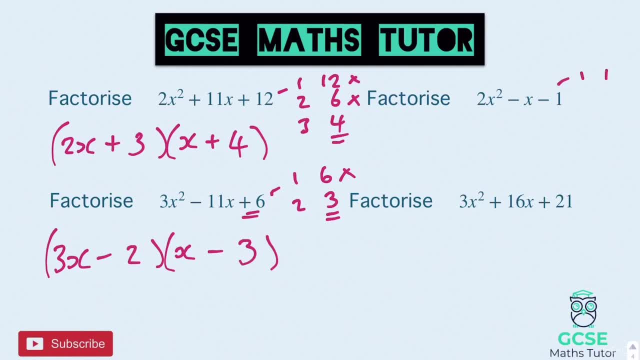 On to this top right. So the only factors are 1 and 1 and 1.. So this is quite a nice one. actually We're going to have 2x and we're going to have x And actually, because our only options are 1 and 1, we can actually stick the 1s in straight away. 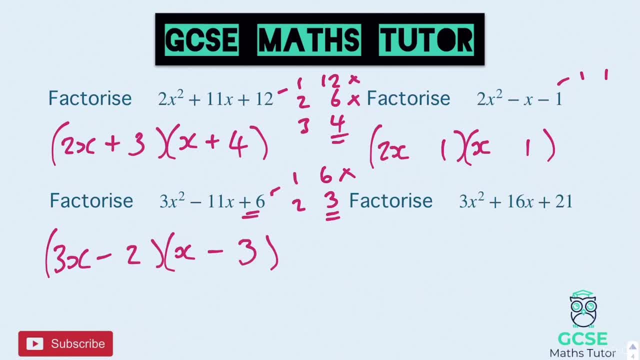 We've just got to get the symbols right here. One of them is going to double, So it's going to be 2 and 1.. So how do I make negative 1 in the middle using 2 and 1?? Well, I want positive 1. take away 2.. 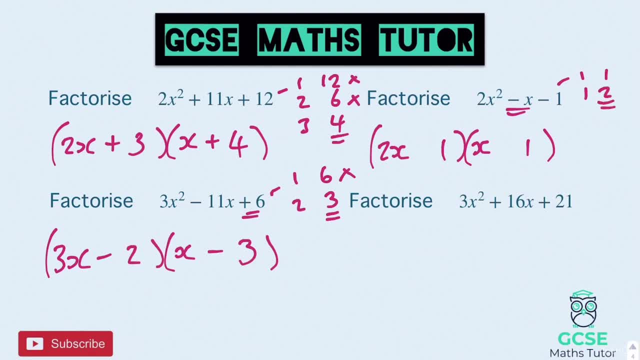 So I want the 2 to double. So let's have a look: 1 and 2, I want the 1 to double to make 2.. So I want positive 1 here. take away 2 in the other bracket. 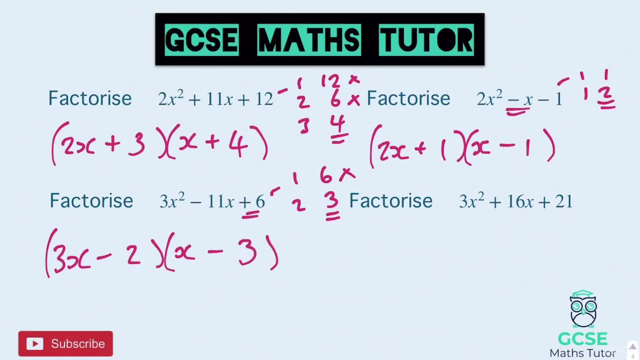 That 1's going to double to make the negative 2.. And on to the last one: 3x squared. So we've got a 3x and an x Factors of 21,. we've got 1 and 21,, or 3 and 7.. 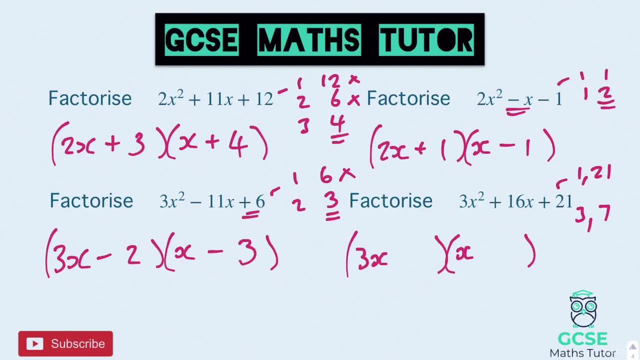 OK, there's my factors, And one of them's going to triple. I'm definitely not going to make 16, tripling that, 21. And if I triple the 1,, that makes 3.. I can make 18 out of that, but I can't make 16.. 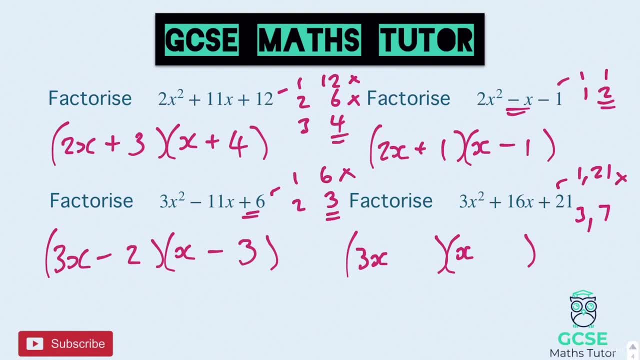 So it's not that one there, So it must be the 3 and the 7.. And let's think which one do I want to triple. I could have 3 tripling to make 9.. And add the 7.. 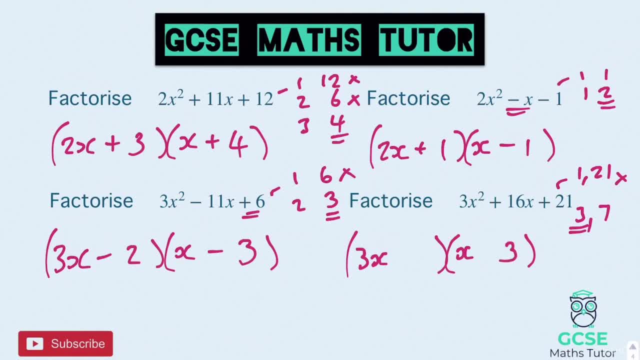 Ah, that works. So there we go. We want the 3 to triple, So we'll stick the 3 in here and the 7 in there, And let's just get the symbols correct. It's all positives, so that's quite nice and easy. 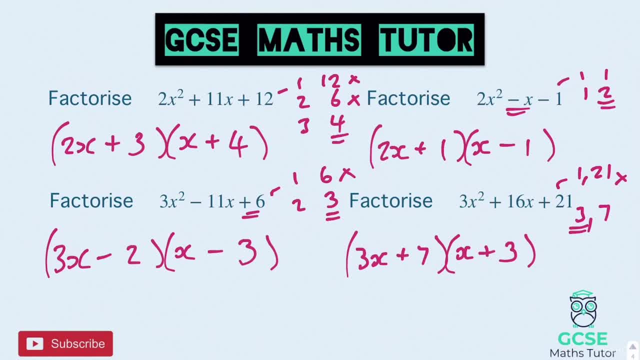 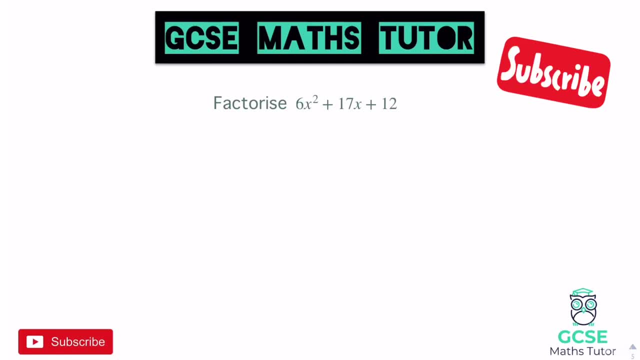 All positives. There we go, And there's factorising some quadratics. Let's have a look at some slightly different ones. OK, so in this question we've got a 6x squared, which means there are different options that we can have in the brackets. 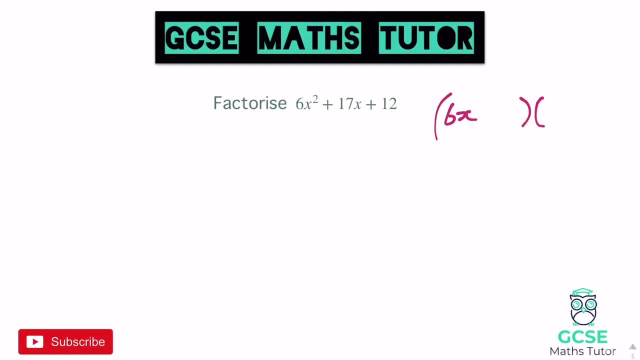 I could have a 6x And a 1x- That would make 6x squared. And I could also have a 2x and a 3x, And that would also make 6x squared. So we've got two options here. 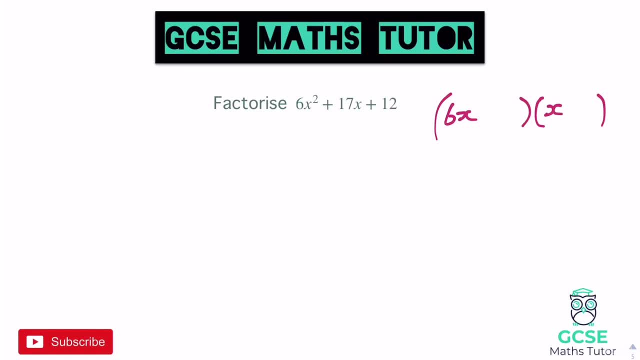 But let's just have a think. I'm just going to go for the 2x and the 3x to start with. So let's just go for the 2x and the 3x And just see if we can make it work. 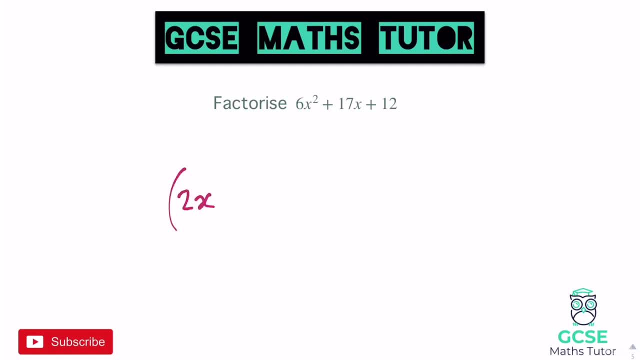 If not, we'll go back to the other one, But let's go with 2x and 3x, OK, So factors are 12.. We've got 1 and 12,, 2 and 6. Or 3x. 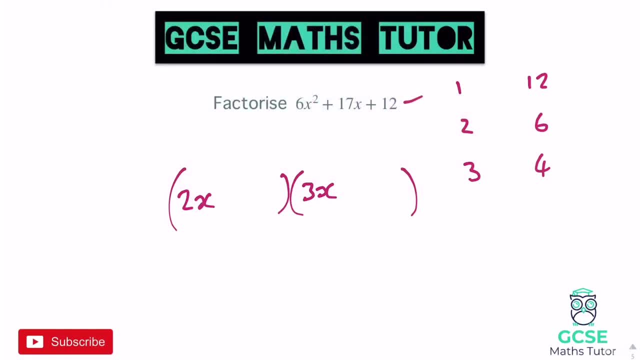 3 and 4.. Now again, this is a little bit harder, Because 1's going to double and 1's going to triple. So you might want to write all the options down, Or you might just want to go about it in your head. 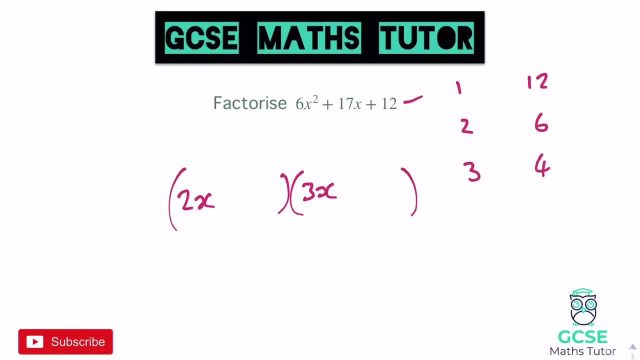 But 1's going to double and 1's going to triple. So if I look at the 1 and the 12., Double 1 is 2.. Triple 12 is 36. We're going way beyond 17.. So that's not going to work. 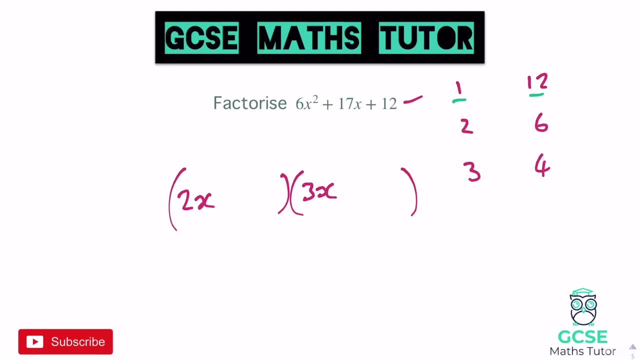 Let's try it the other way around. Triple the 1 is 3.. Double the 12 is 24.. 24 and 3.. Again, I can't make 17.. So it's not that one. Let's go for the 2 and the 6.. 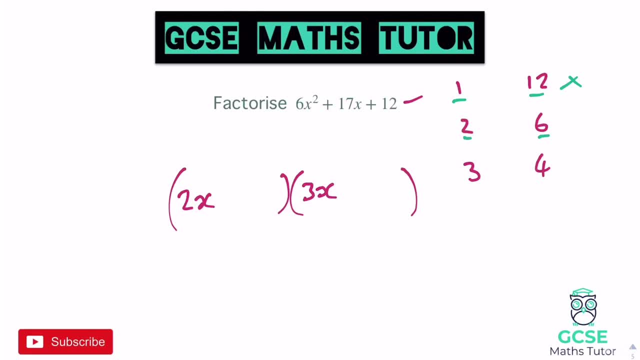 Double 2 is 4.. Triple 6 is 18.. So 4 and 18.. That's not going to make 17.. Try it the other way around. Triple the 2 is 6.. Double the 2 is 12.. 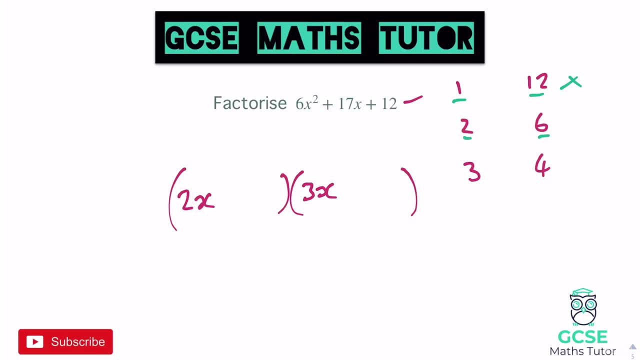 So 6 and 12. I can only make 18.. I can't make 17.. So it's not that one, It's going to have to be 3 and 4.. So let's have a look, Let's just write these ones down. 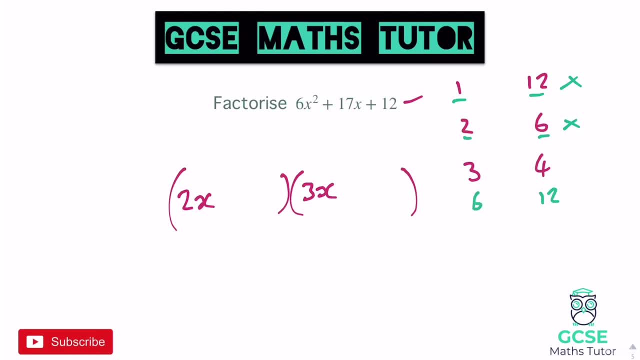 So double the 3 is 6.. Triple the 4 is 12.. Or triple the 3 is 9.. Double the 4 is 8.. Which option there makes 17?? It's the 9 and the 8.. 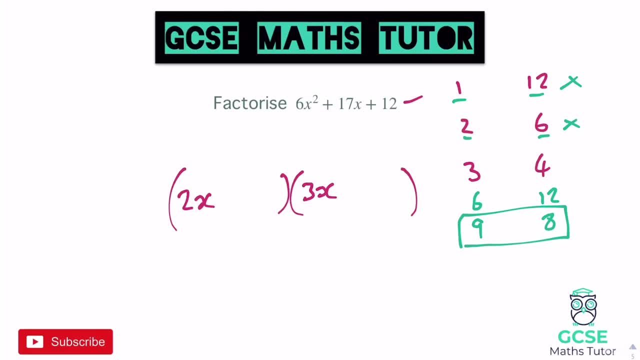 So I want the 3.. I want the 3 to be tripled, So I need to put that in the opposite bracket to the 3x. So 3 is there And I want the 4 to be doubled, So that's going to go in this bracket. 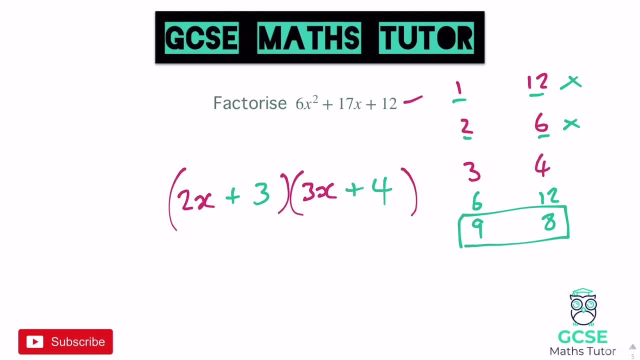 And again it's all pluses. So all positive symbols there: 2x plus 3 and 3x plus 4.. You've just got to take your time with these. Really, think about those factors, Write down as much as you need to to make that work. 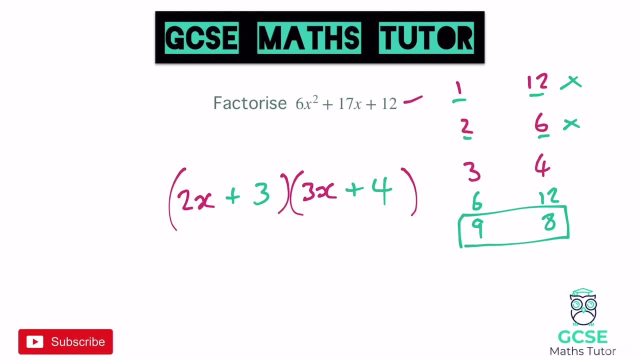 Again, the better you are with numbers, the more easy you'll find this doing it in your head, But otherwise, do write down everything there to the side. Let's have a look at one more. Okay, so we've got a 9x squared. 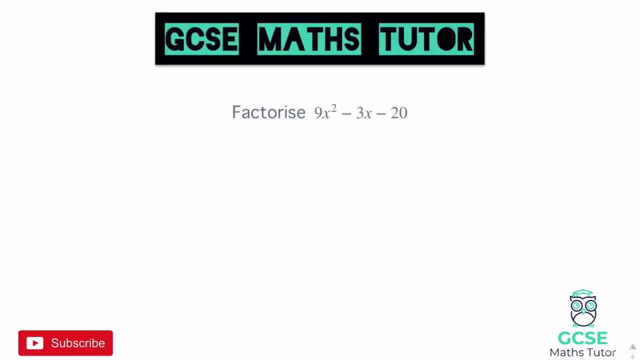 And this one 9x squared is not too nice here, But I'm going to go for 3x and 3x again. We could have 9x and 1x, But let's just try this one out: 3x and 3x. 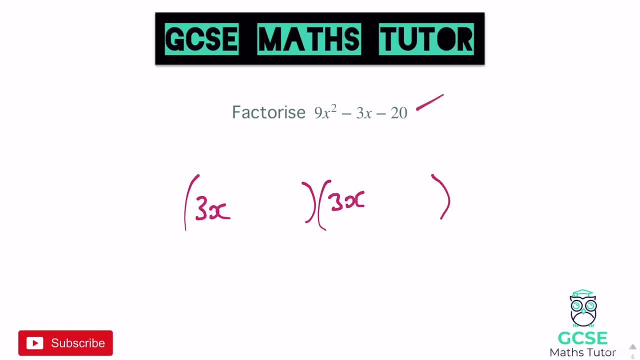 Which means both of my factors this time are going to triple. So what factors have we got? We've got 1 and 20.. Very unlikely to be that one, Because I don't think we're going to make negative 3 if we're getting 60 in there in one of the factors. 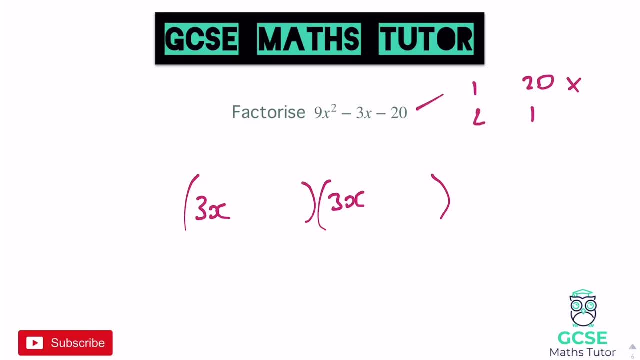 So, straight away- I know it's not that one- We could have 2 and 10.. Unlikely that we're going to be using 30. But let's have a look And we could have 4 and 5.. Now, because there's a negative 3 in the middle. 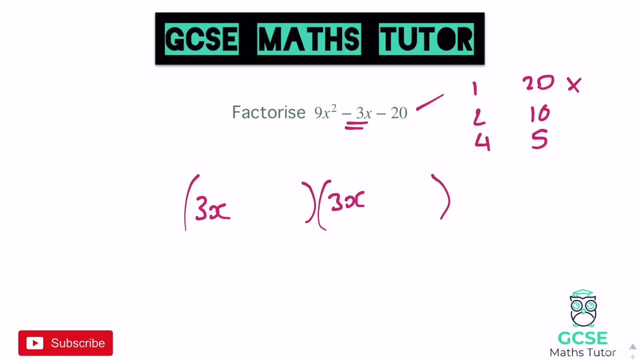 I'm going to think it's probably not the 2 and the 10. Because that's very close to 0. So I'm going to imagine the numbers are quite close together. But 2 and 10, let's just have a quick think. 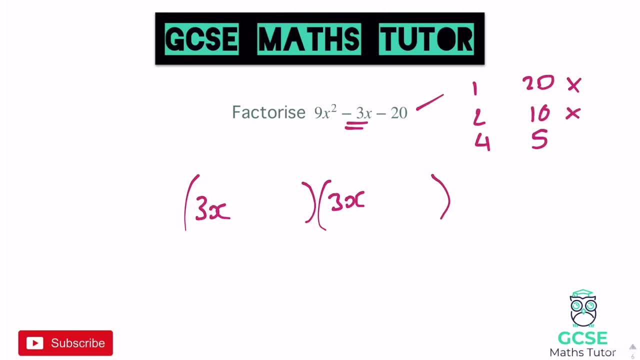 That would be 6 and 30.. No, we're not going to make negative 3.. So it's got to be the 4 and the 5.. So let's just have a quick think: If we triple them, at least they're both being tripled. 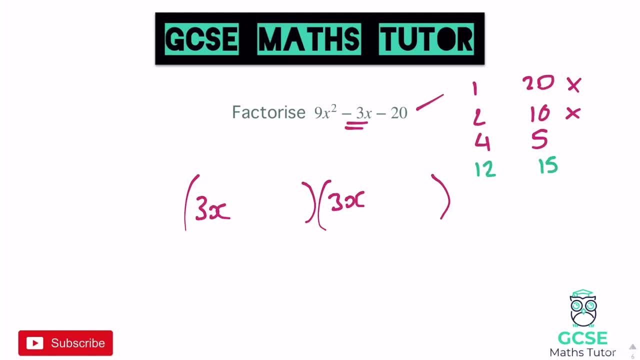 So it's 12 and 15.. It's my only option. And how am I going to make negative 3 out of that? I want positive 12.. And I want negative 15.. Okay, so I want the 5 to triple as a negative. 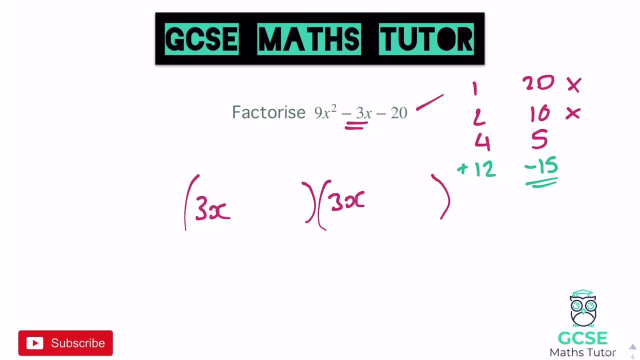 Because I want negative 15.. So I want to put negative 5 in the Well, because they're both 3, either one, So negative 5.. And I want positive 4 in the other one. That's going to allow me there to get that. 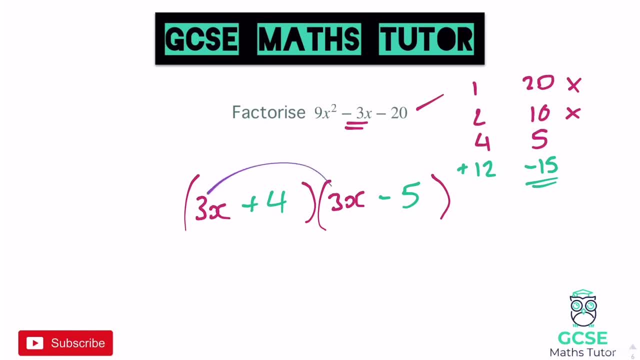 And you can always again just check to expand it. So 3x times 3x is 9x. squared, 3x times negative, 5 is negative. 15x. 4 times 3x is 12x. 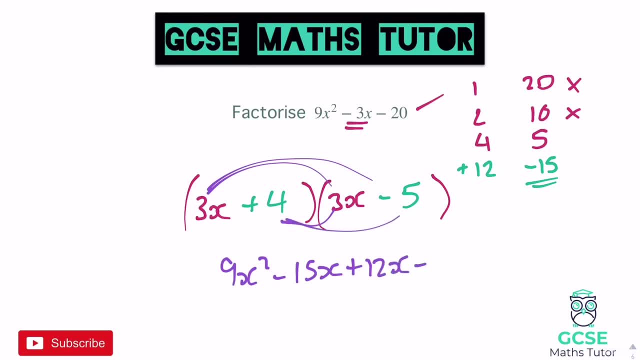 So plus 12x And then 4 times negative, 5 is negative 20. And again, you can just simplify these And you get 9x squared, 9x squared minus 3x minus 20.. There we go. 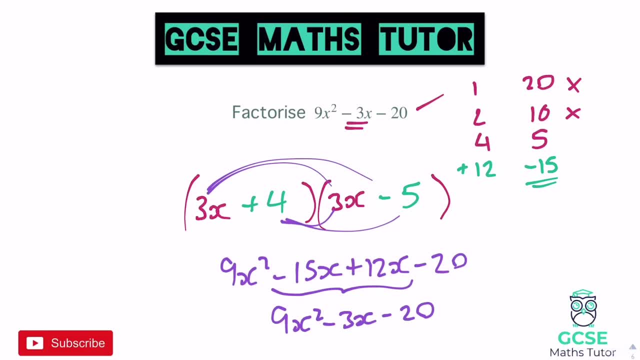 And that is expanding or factorising- sorry- a quadratic where the coefficient is bigger than 1.. And we have different options here with the numbers that could go into the brackets. So too few to have a go at Here. they are Okay. so here's your two questions. 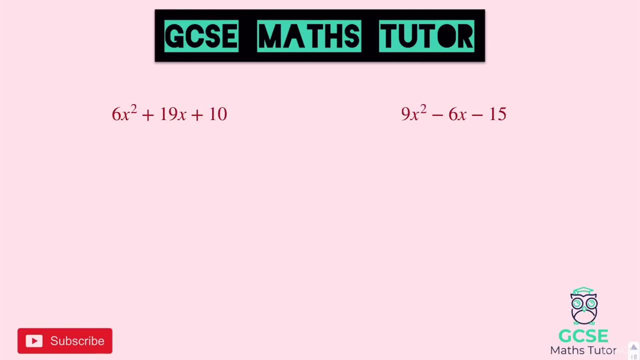 Pause the video there. We'll go over the answers in a sec, Okay. so, looking at these two, So we'll go for 2x and 3x for this first one. Okay. So 6x squared there And let's just write down the factors of 10.. 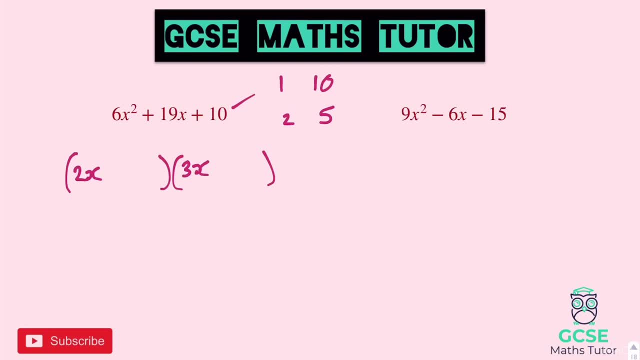 So we've got 1 and 10 or 2 and 5.. Now 1's going to double, 1's going to triple. So if we think about this, if we double the 1, we'll get 2.. 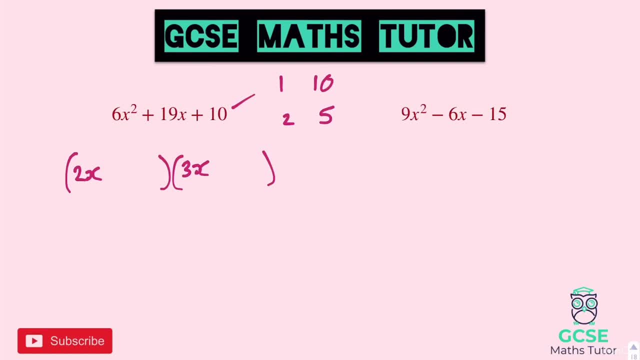 Triple the 10 is 30. That's not going to work. Triple the 1 would be 3.. Double the 10 is 20.. So we can make 17 or 23,, but not 19.. So that's not going to work. 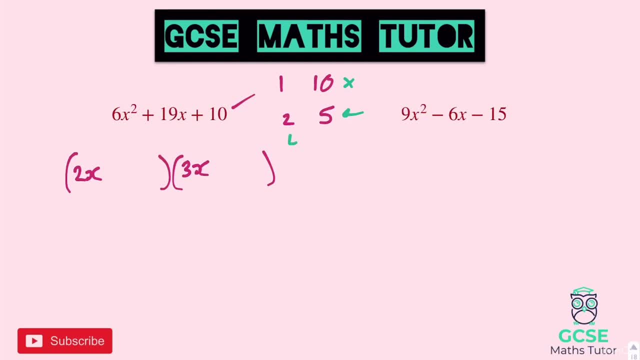 And so it must be the 2 and the 5.. So if we double 1, we'd get 4.. Triple the other is 15.. Or triple the 1 is 6 and double the other is 10.. So to make 19,. we're going to need that 4 and 15 there. 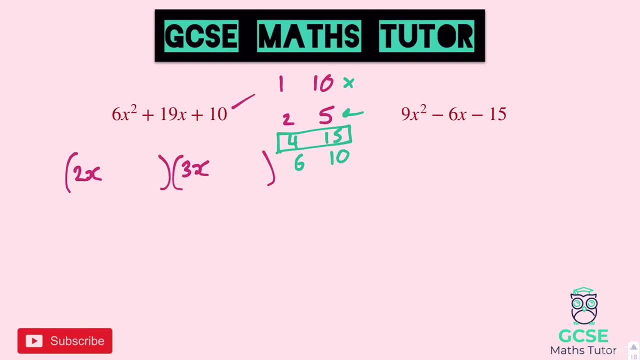 And they're both positive. We want the 2 to double and the 5 to triple. So if we want the 2 to double, we stick it in the opposite bracket to the 2. And we want the 3 to triple. 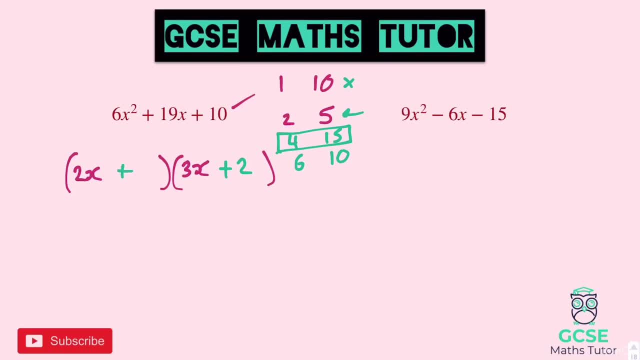 Sorry, the 5 to triple. So stick that in the opposite bracket to the 3.. So plus 5.. So there's that one factorised On to the other one. We've got 9x squared. Let's go for 3x and 3x again.